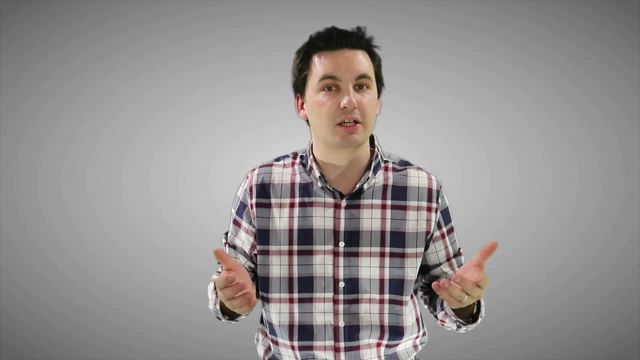 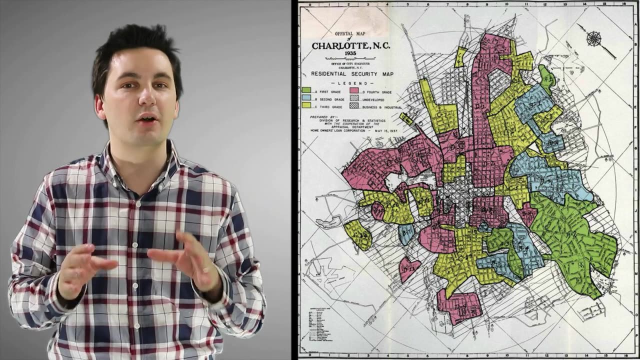 These communities were often minority communities and redlining allowed people to move out of their neighborhoods, As communities that weren't located in a red district were allowed to get cheaper loans- traditionally white communities. this allowed them to be able to purchase a home and eventually resell it and pass wealth down through the generations. While communities that were located in redlined neighborhoods were not able to get these loans and were not able to move out. this continued the segregation of America, and it also led to a generational gap in wealth, as communities again that weren't redlined were able to sell their homes and buy a new home. 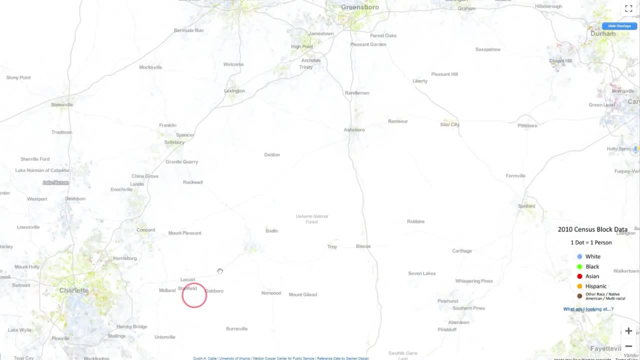 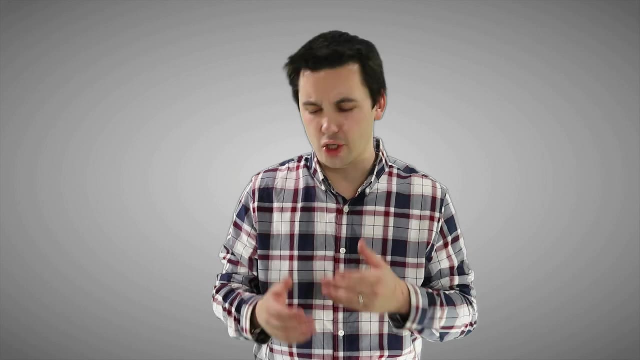 and pass down wealth through the generations. Now that the redlining isn't practiced anymore, the damage is done and we can still see the impact of these policies when looking at our cities today. And it wasn't just redlining that's further segregated our neighborhoods. We could also look at the impact of blockbusting, which happened in the 50s and 60s. This was when real estate agents would go into white communities and convince them to sell their homes to the real estate agents at a cheaper rate. They would use the fear of minority communities moving into the neighborhood and the risk of losing property value. These real estate agents would then sell the homes to the people who were living in the neighborhoods to minority communities at a higher rate. This led to white flight and continued to segregate neighborhoods throughout the United States. 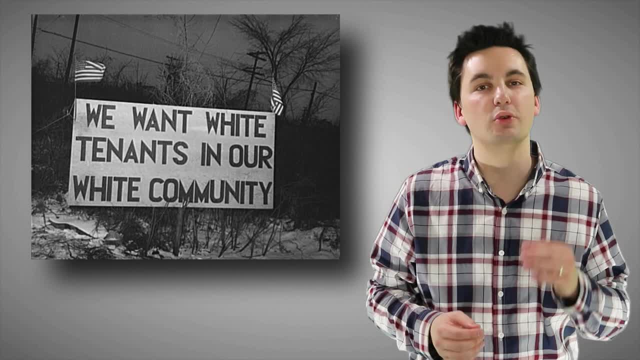 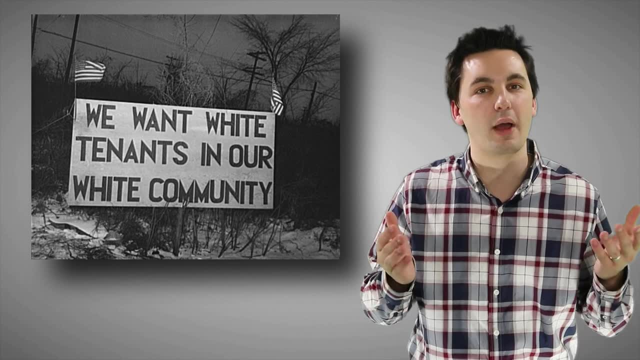 White flight was the migration of white communities out of a city due to minority communities moving in. This led to the further segregation of neighborhoods, both racially but also economically. This is where we started to also see the formation of ghettos, inner city and segregated neighborhoods. 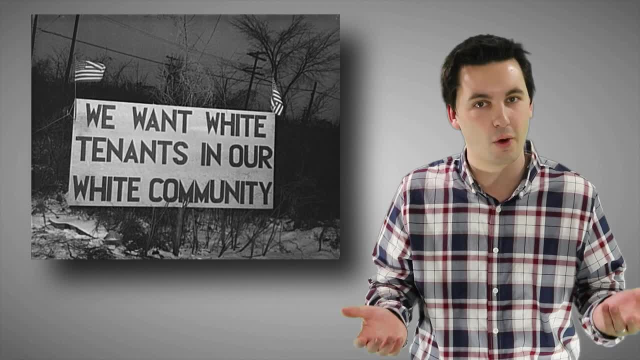 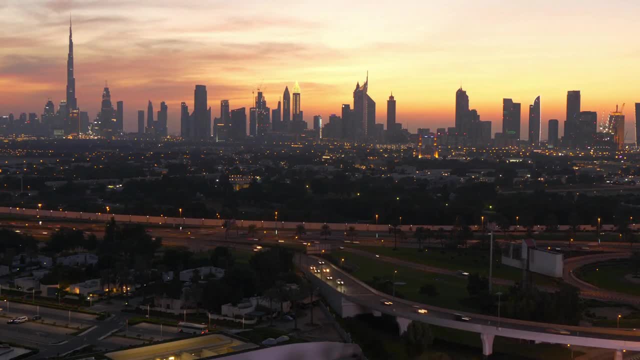 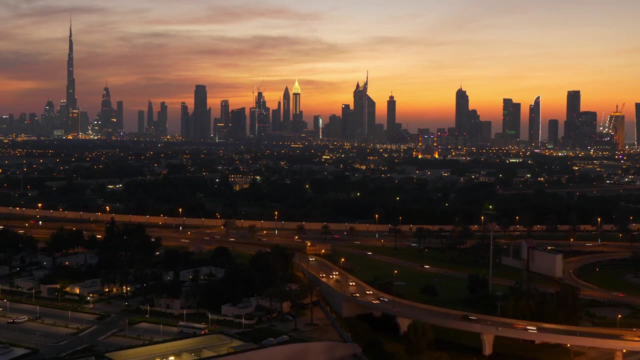 that disproportionately favored white communities over minority communities. We can see that segregated cities often struggle with providing economic and social opportunities for all residents. These cities will often see resources disproportionately favor wealthier communities. Parts of the city that have less affluent residents are more likely to have higher crime rates. 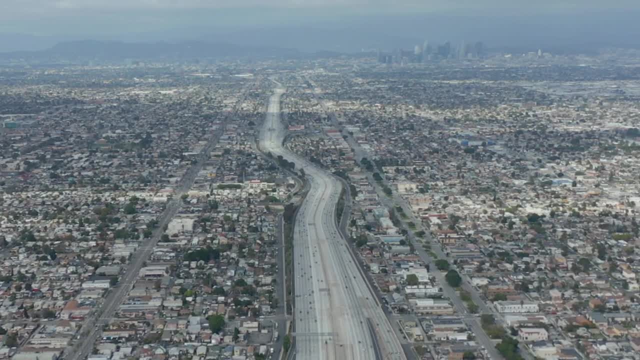 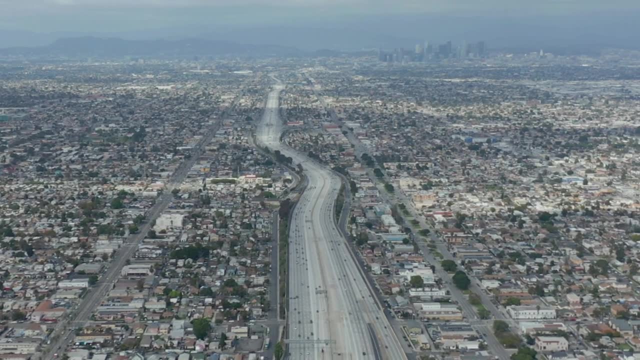 less job opportunities, less access to important services like health care or education, and they're more likely to see more pollution and also experience more urban blight, also known as urban decay. Today, if we look at large urban areas and also some rural areas, 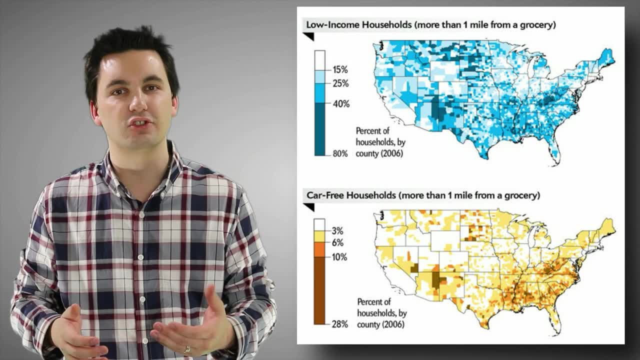 we can see that there are a lot of urban areas that are more likely to experience urban decay. We can also see the impact of food deserts, which creates unique challenges for settlements. Individuals living in a food desert traditionally are more likely to be low income. 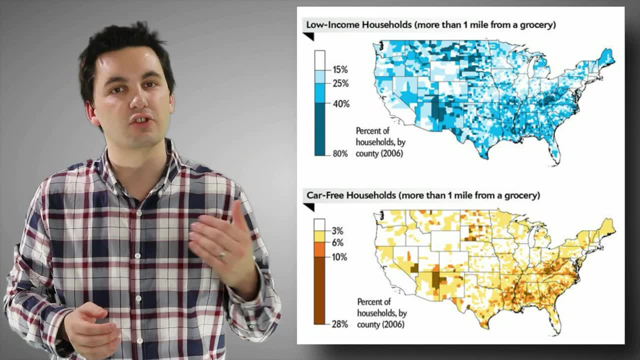 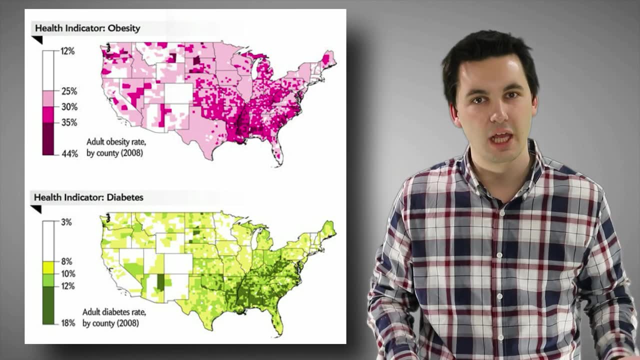 have health concerns and are not going to be able to get access to fresh food and healthy food. Residents in a food desert depend on fast food and also convenience stores in order to get food. Here we can see that options are scarce and residents are more likely to experience diabetes and obesity. 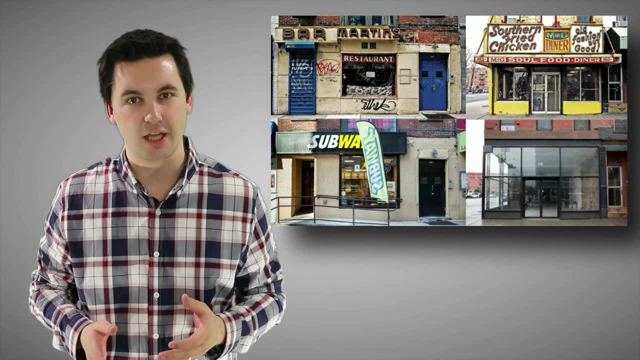 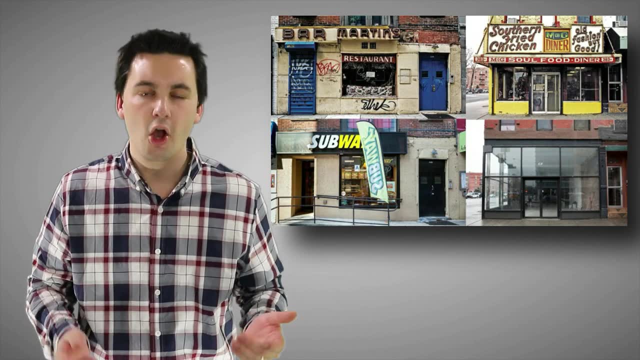 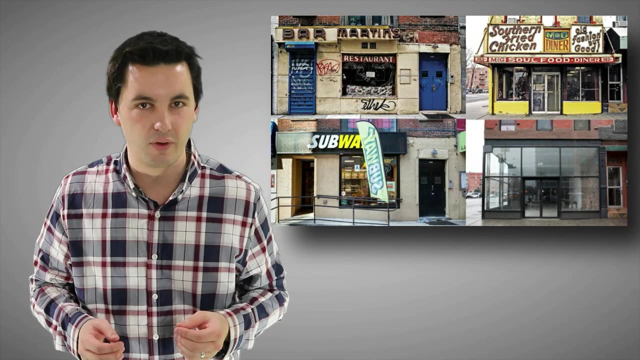 Speaking of low-income areas, we can also see the impact of gentrification. This is when middle-class residents move into low-income areas traditionally located near the CBD. Often times, these middle-class residents are single and they're looking to gain access to the goods and services that the CBD provides. 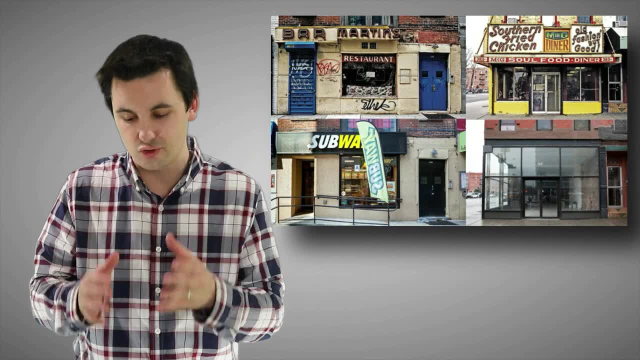 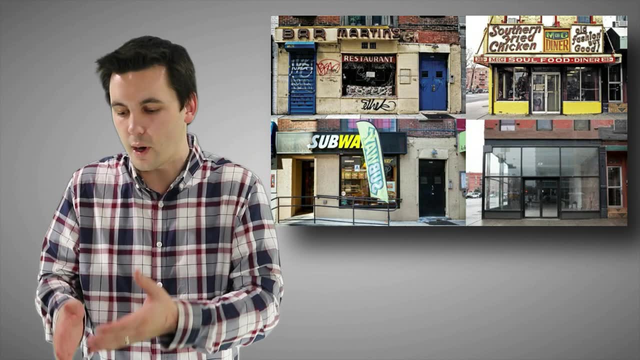 They also might be moving there because they have a unique connection to the historical architecture or that community feel. When they move into these low-income areas, though, they renovate the homes. they convert warehouses into stores or apartments. This increases the value of land in that community. 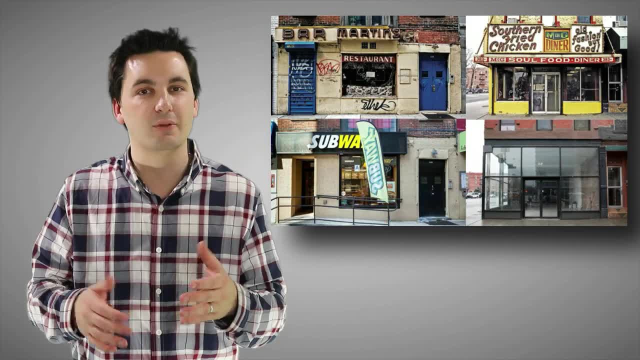 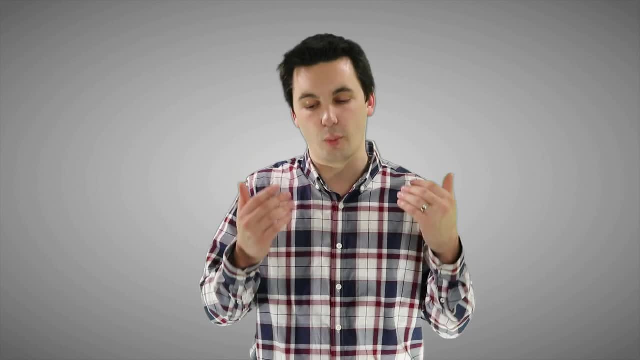 This increases the value of housing in that neighborhood, causing rents to go up and also possibly taxes. We can see this has created kind of an interesting debate. On one hand we can see that gentrified neighborhoods will attract more businesses, goods and services. 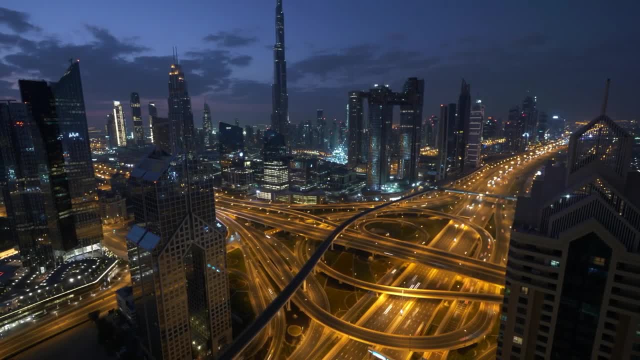 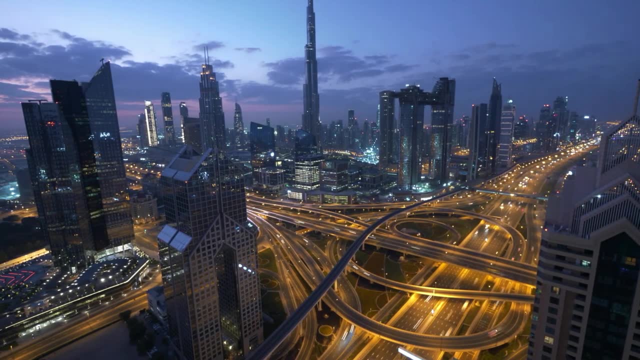 We'll see more wealth move into the area. This can create more economic opportunities and also social opportunities. All of this will attract more investments and people into the neighborhood, which can benefit the economic development of the neighborhood and also the opportunities for residents. But on the other hand, we could also see that people who are living in low-income areas will see some negative effects as well, as we might see those rents increase and taxes increase, which will push out the low-income residents that were originally living in the neighborhood, causing displacement to occur. This could lead to more homelessness or also a shortage of homes for people who have less wealth. 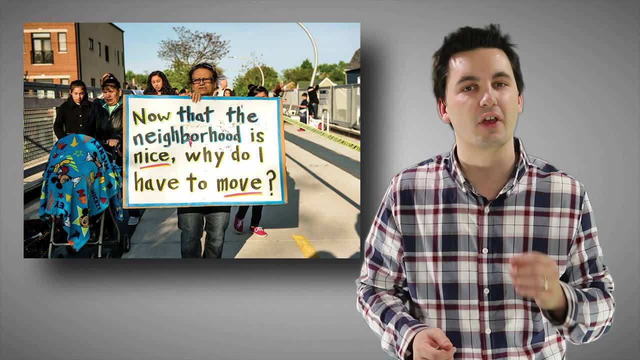 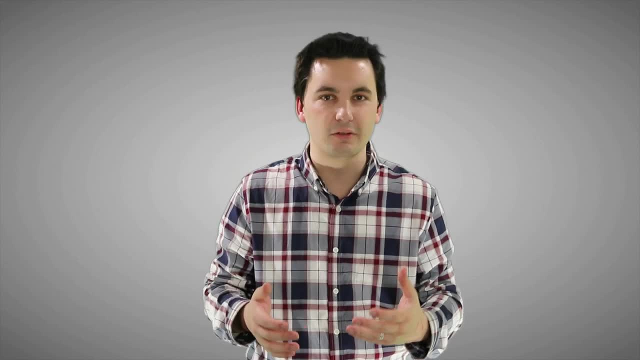 Again favoring then the middle class and wealthier residents of the neighborhood. Another challenge that cities and settlements can face is the different layers of government and their involvement in city planning, regulation and also funding. The federal governments may see the federal government get involved in city planning. 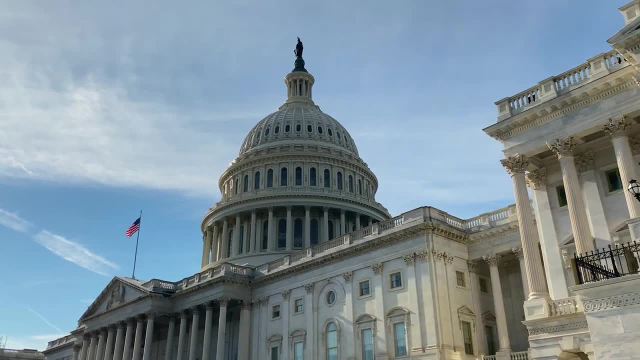 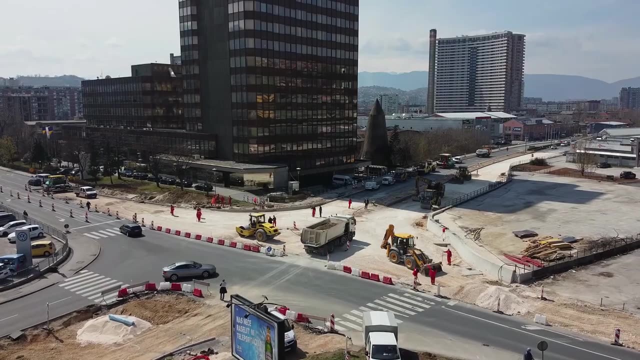 However, in countries like the United States, the federal government is not allowed to do any city planning. However, we can still see the federal government influence city planning and infrastructure projects by giving funding to cities and states for projects and adding special guidelines to the use of that funding. 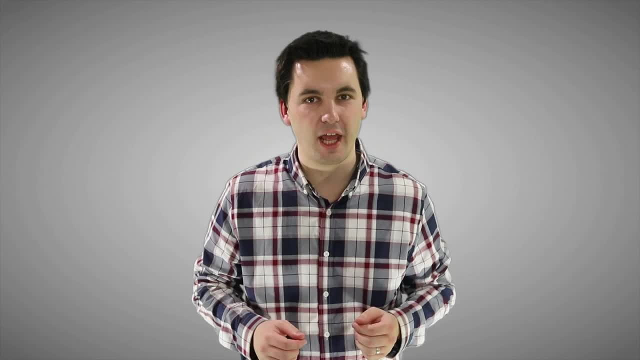 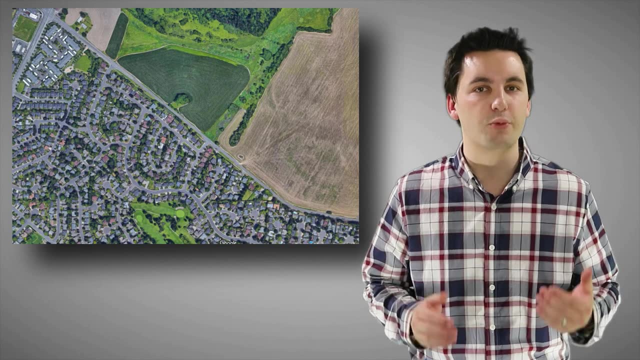 If we look at the sub-national level, for example, state governments in the United States, we can see that government does play a role in urban planning. For example, if we look at the state of Oregon, we can see that the state sets growth boundaries for urban areas. This protects the farmland and the rural communities by preventing urban sprawl from occurring. It also increases the density for cities as there is measures put in place to prevent sprawl from happening, containing the urban areas in set spots. We can also see the impact of local governments with cities and counties. Cities are able to zone and rezone parts of the city, They set the budgets and they have a lot of influence on the day-to-day lives of their residents. Counties, on the other hand, take care of the unoccupied territory between the different settlements within the county's boundaries. All these different levels of government allow for more specialization to occur and allow us to focus our city planning more regionally. At the same time, you can see how this could create challenges. If the federal government wants to create certain projects, they may have strings attached. 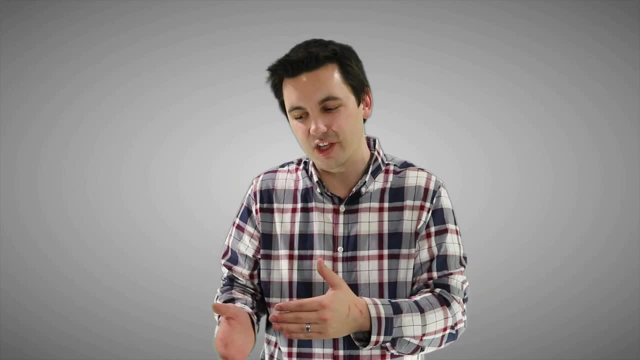 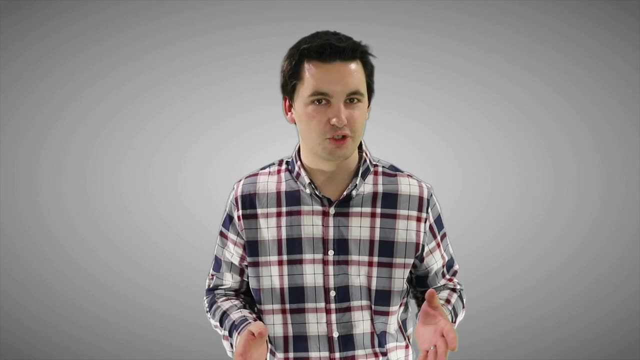 If the states have an idea for what they want for the state and the cities disagree, we could see some conflict And unfortunately, sometimes this bureaucracy can slow things down or make cities a little more inefficient. And we didn't even talk about special districts. 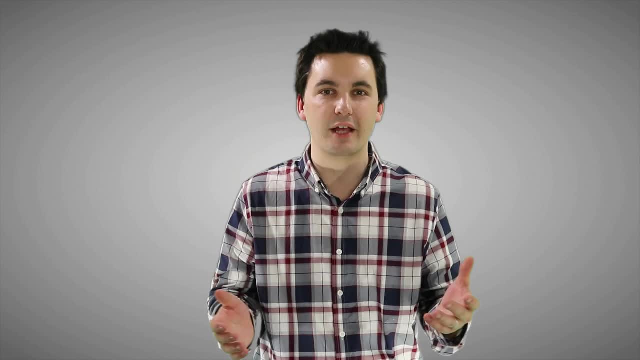 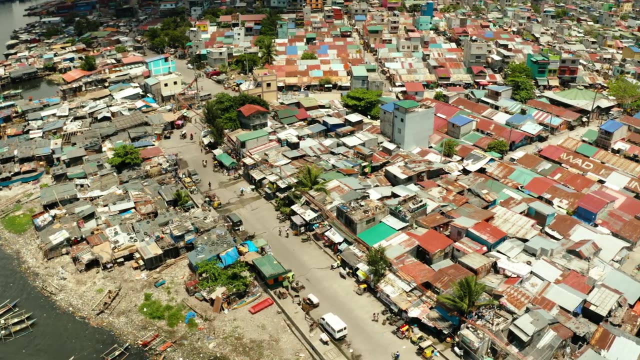 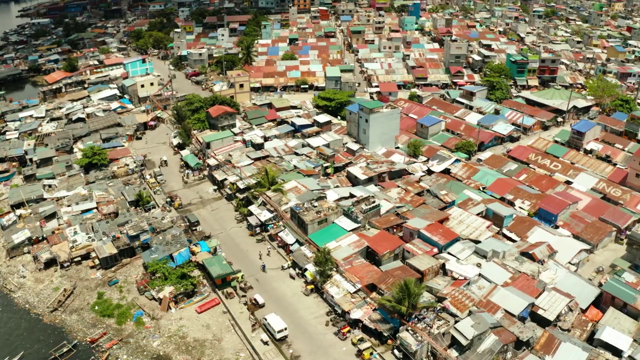 which are units of government that provide specific services for residents. Now, if we expand the scope of our conversation, we can also see cities around the world, especially in the periphery countries, are struggling with squatter settlements, Oftentimes when cities are seeing rapid population change and lack affordable housing. 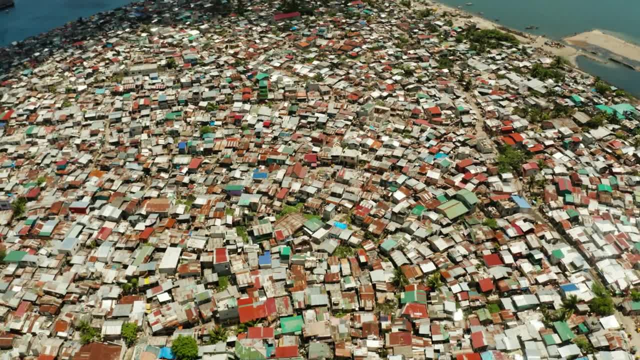 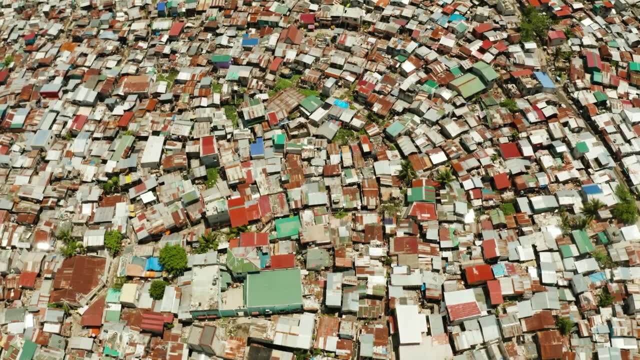 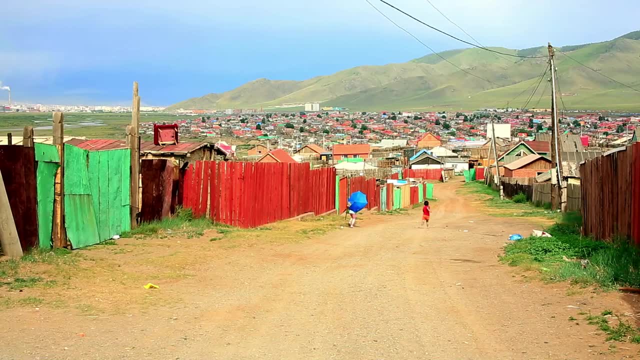 we start to see the formation of these settlements occur. Squatter settlements are areas in which residents have developed on the land without actually having a legal claim. These areas will often lack essential services like water, electricity, sewage, medical care, education and other important infrastructure. 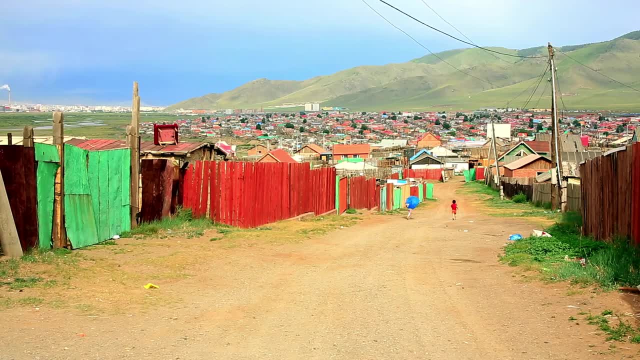 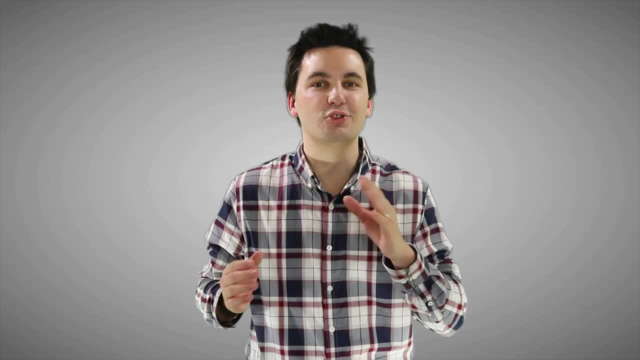 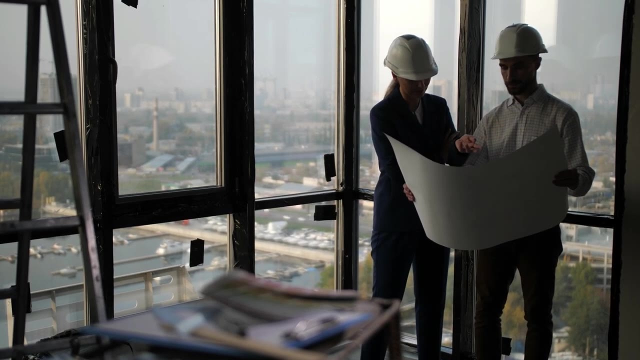 And they're more prone to seeing high amounts of crime and poverty. All of this creates unique challenges for these cities as they try to adapt to the changing population. As we can see, cities struggle with a variety of unique challenges, And when cities are up to the challenge and utilize urban planning and work to continue. to adapt to the needs and wants of the city, they're going to have to face a lot of challenges. And when cities are up to the challenge and utilize urban planning and work to continue to adapt to the needs and wants of the city, they're going to have to face a lot of challenges. 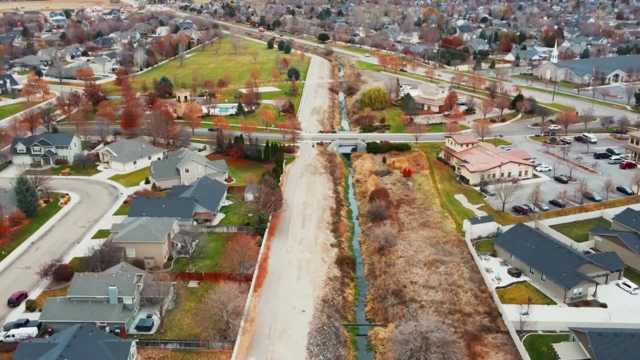 And when cities are up to the challenge and utilize urban planning and work to continue to adapt to the needs and wants of the city, they're going to have to face a lot of challenges In a sustainable manner, we can see cities thrive. However, we can also see the impact when cities fail to do this. 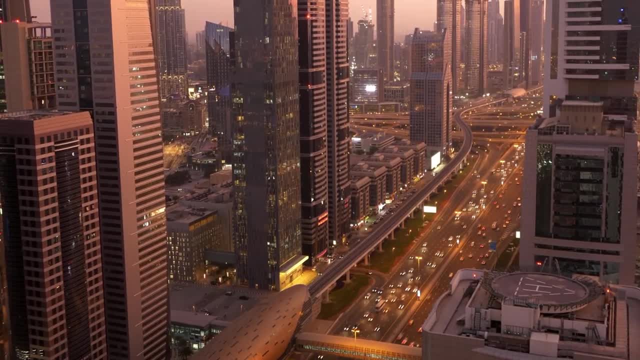 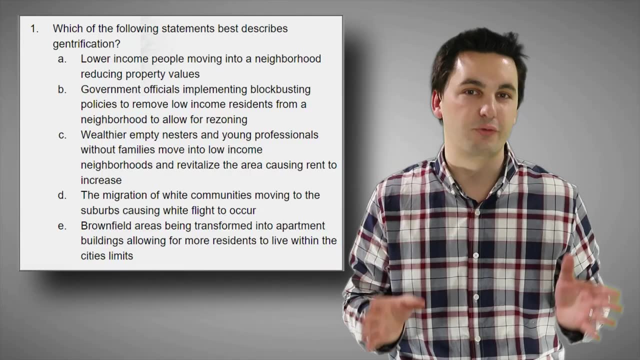 And as we continue to see our population change in the world and more migration happen, we'll continue to see new challenges brought upon cities around the world. But now we're getting into the future And instead of talking about the future, we need to talk about the present. 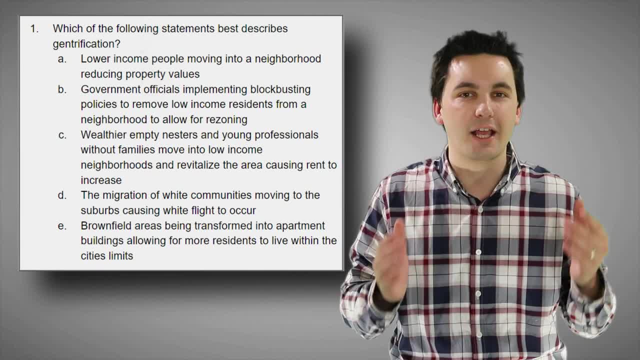 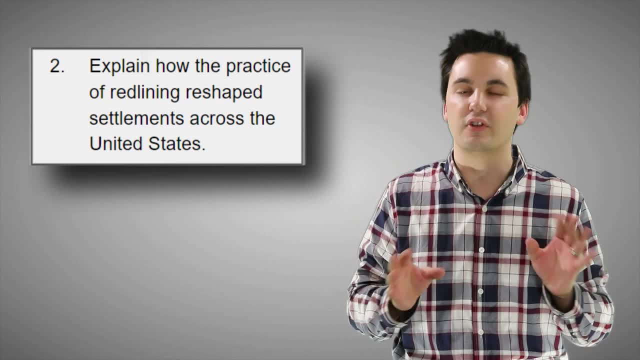 And we need to now review what you've just learned. Take a second and answer the questions on the screen right now. When you're done and you think you got the answers, check them down in the comments below. Once you've checked your answers and you made sure you've got all the information set. 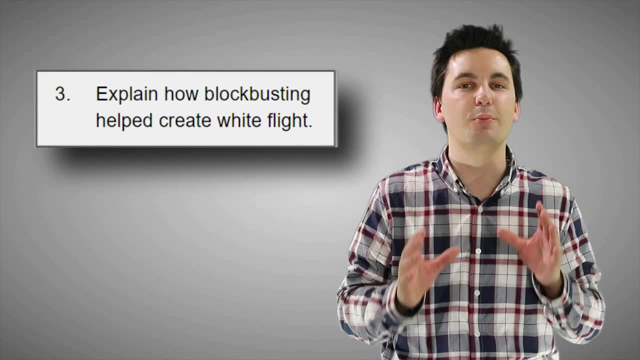 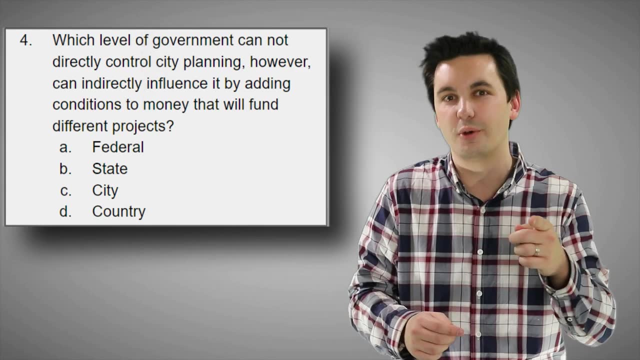 don't forget to hit that subscribe button and share the video. It helps support the channel and it allows me to keep making more topic review videos for you guys. Plus, you'll never miss out on any of the future videos, so you'll always be up to date for your class. 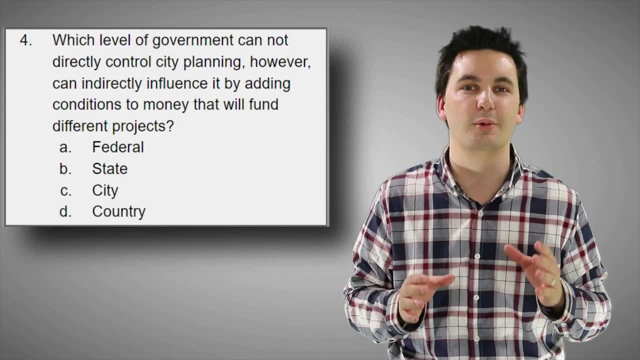 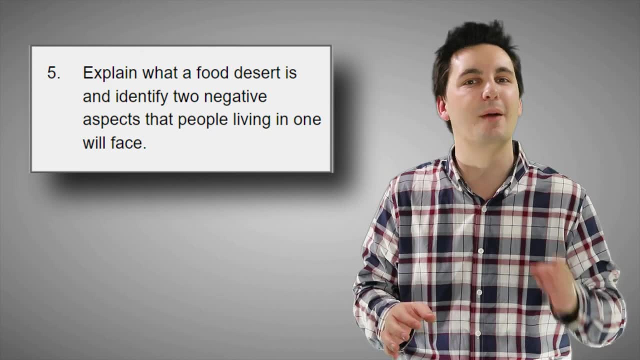 And if you are struggling with AP Human Geography, don't forget to check out my ultimate review packet. You can find a link in the description below. All right, Thanks so much for watching geographers. I'm Mr Sin, And until next time I'll see you guys online. Bye. 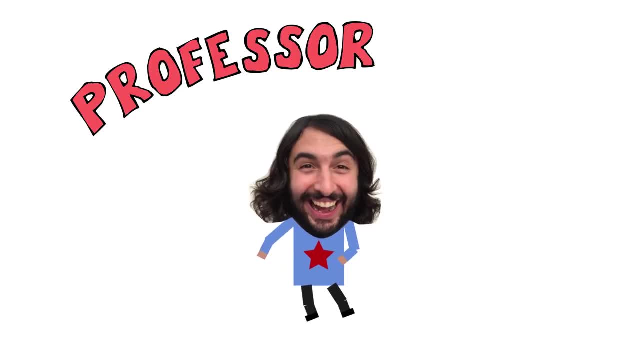 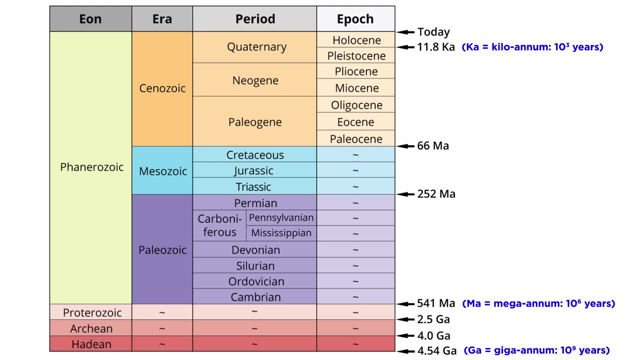 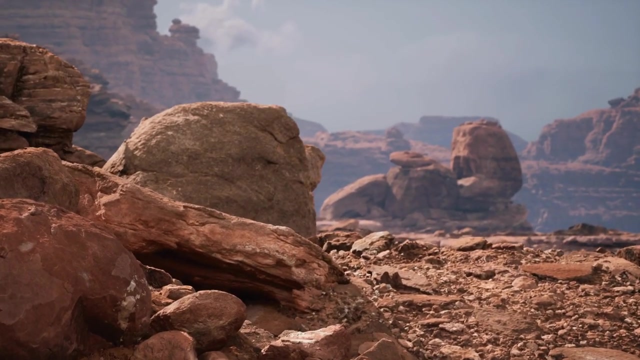 We just got finished discussing the four eons of geologic time, those being the Hadean, Archean, Proterozoic and Phanerozoic. Now let's get more specific with the geologic structures that span those eons. We're going to explore how rocks on Earth.